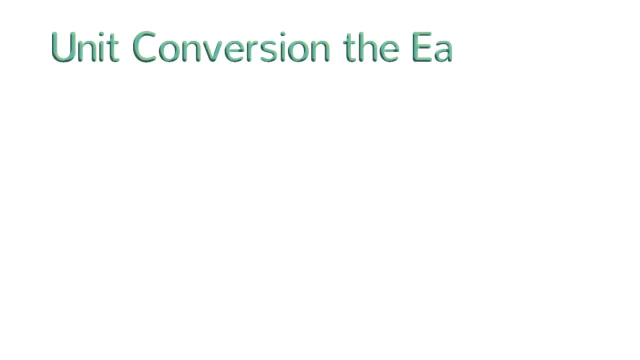 Learn unit conversion the easy way. The method that we will be using to convert between units is known as dimensional analysis, or the factor label method, or even the unit factor method, But what we call it really doesn't matter. What matters is the fact that this is a versatile and 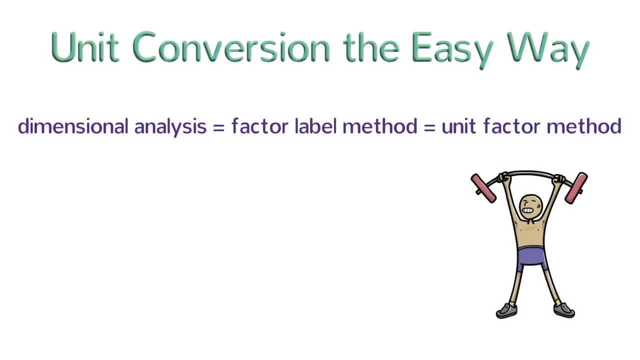 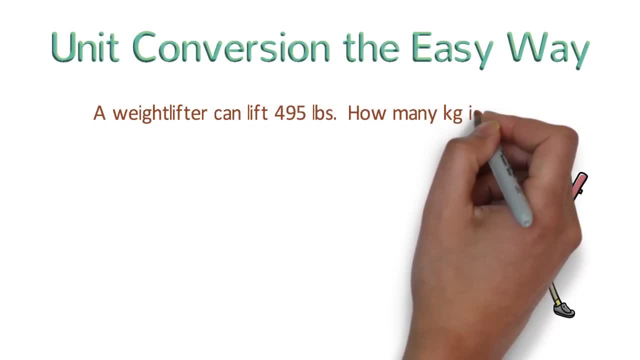 powerful problem solving technique, So let's just do this. We're going to start with a simple unit conversion problem. A weightlifter can lift 495 pounds. How many kilograms is that? In order to solve a unit conversion problem like this, we first need one more piece of information: the 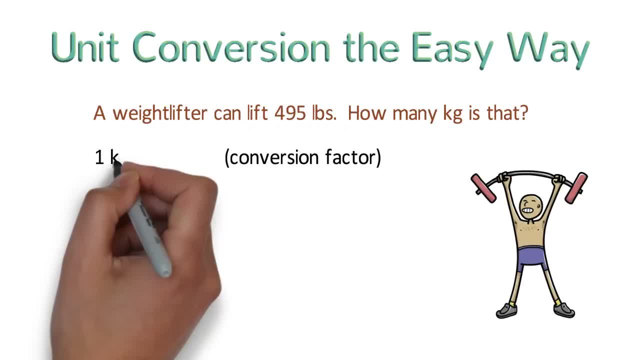 conversion factor For pounds and kilograms. the conversion factor is: 1 kilogram equals 2.2 pounds. Now we're ready to solve this. The first thing you should always do is write down the quantity that you want to convert. This is the number from the question, not the conversion factor, Please. 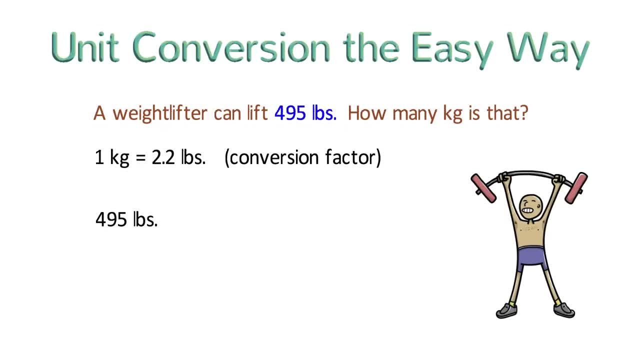 also include the units. Next, we're going to multiply this number by a fraction. Inside the fraction, we're going to multiply it by a fraction. We're going to multiply it by a fraction To write the two numbers from the conversion factor. But how do we know which one goes on top? 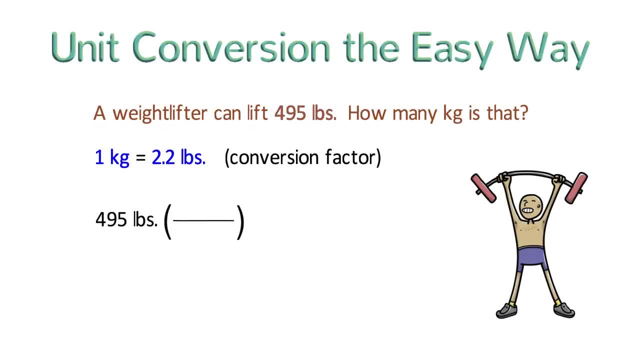 and which one goes on the bottom? To answer that question, all we need to do is look at the units, which is why we always include the units in the calculation itself. The quantity we are starting out with has the units of pounds. So we take 2.2 pounds from the conversion factor and write it on. 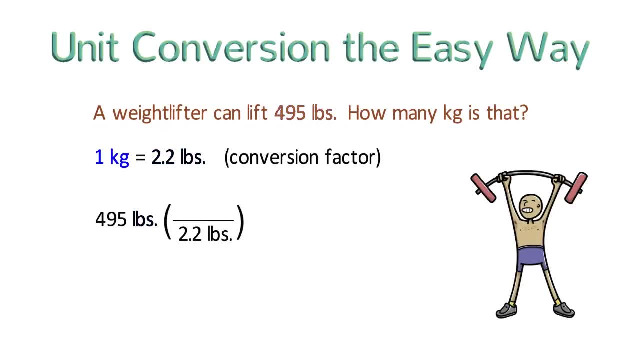 the bottom. Next, because we want to end up with kilograms, we take one kilogram from the conversion factor and write it on the top of the fraction. Notice that the pounds that we started out with cancel out with the pounds on the bottom And the. 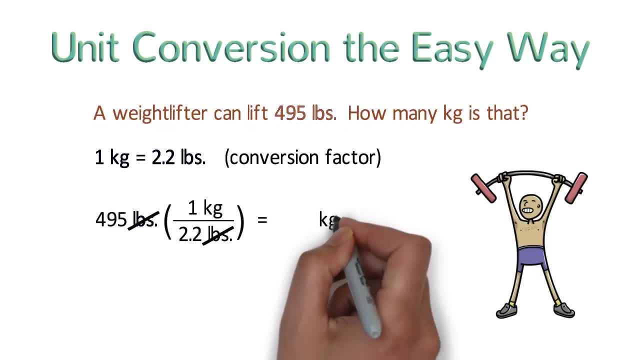 units that we have left on the top are kilograms, which is exactly what we want to convert to. The only thing left to do now is plug the numbers in our calculator. You could, of course, put this in your calculator exactly the way it appears here, But maybe you don't have one of those fancy. 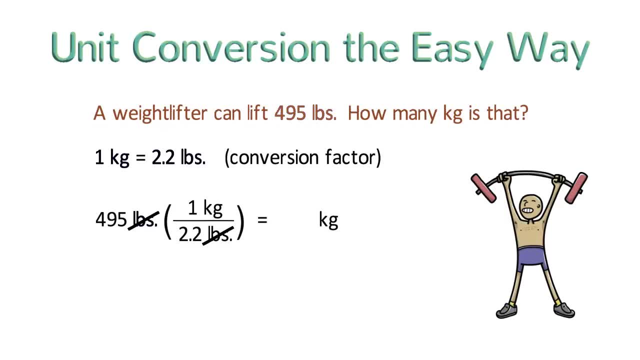 calculators that can do fractions, Or maybe, like me, you just want to find a shortcut, Because the number on the top of the fraction is one. this becomes a simple division problem. In your calculator type, 495 divided by 2.2, and your calculator should tell you the answer is 225.. Our 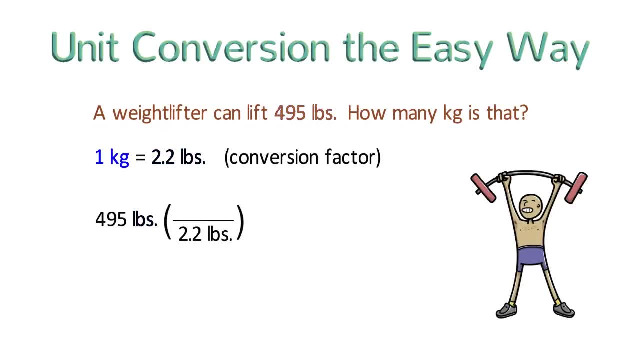 the bottom. Next, because we want to end up with kilograms, we take one kilogram from the conversion factor and write it on the top of the fraction. Notice that the pounds that we started out with cancel out with the pounds on the bottom And the. 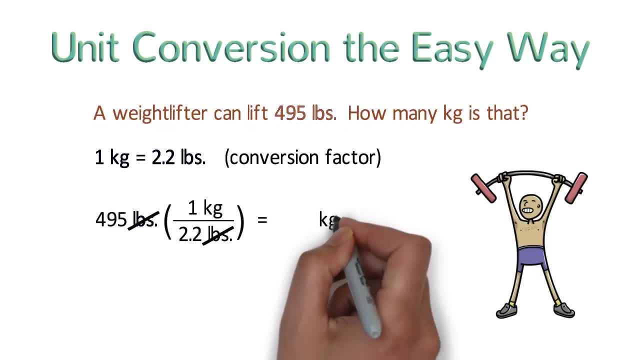 units that we have left on the top are kilograms, which is exactly what we want to convert to. The only thing left to do now is plug the numbers in our calculator. You could, of course, put this in your calculator exactly the way it appears here, But maybe you don't have one of those fancy. 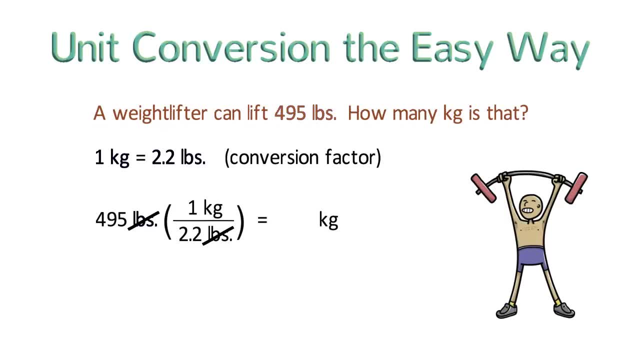 calculators that can do fractions. Or maybe, like me, you just want to find a shortcut, Because the number on the top of the fraction is one. this becomes a simple division problem. In your calculator type, 495 divided by 2.2, and your calculator should tell you the answer is 225.. Our final 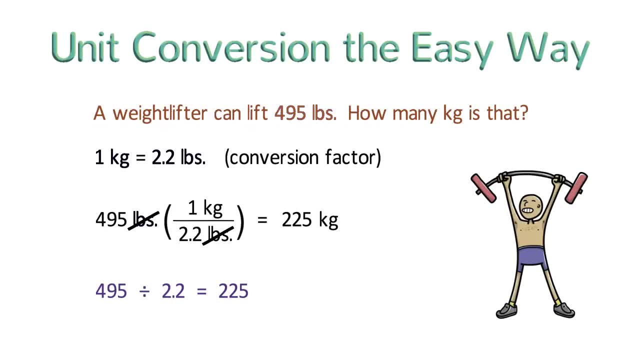 answer, therefore, is 225 kilograms. There is one more thing that we should notice about this problem: The fraction 1 kilogram over 2.2 pounds actually equals 1, because 1 kilogram equals 2.2 pounds, In fact, anytime. 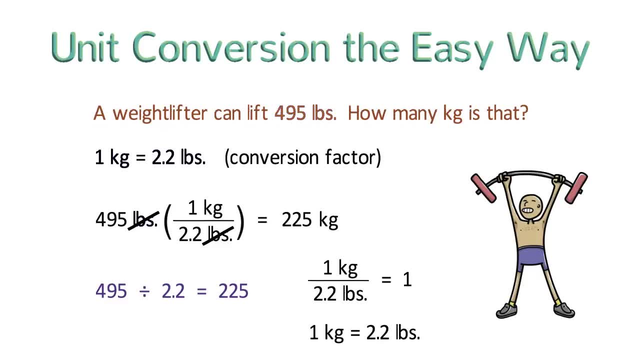 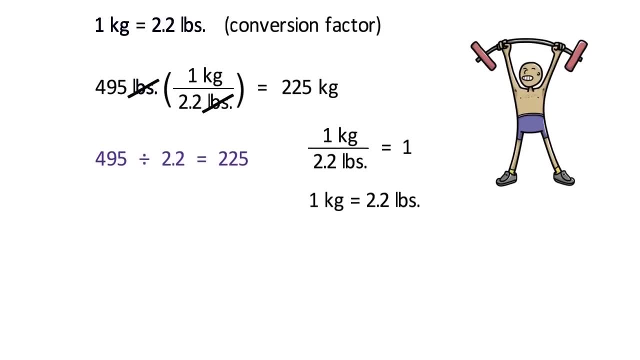 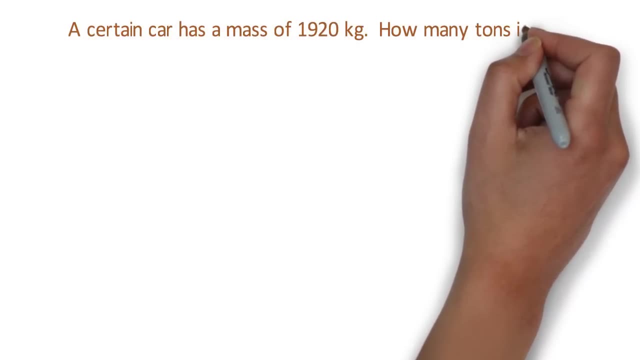 we do unit conversion. we are simply multiplying our initial quantity by a conversion factor fraction that equals 1.. Okay, Now that we are experts at this technique, let's try a slightly harder problem. A certain car has a mass of 1920 kilograms. How many tons is that? Just like always, we need a 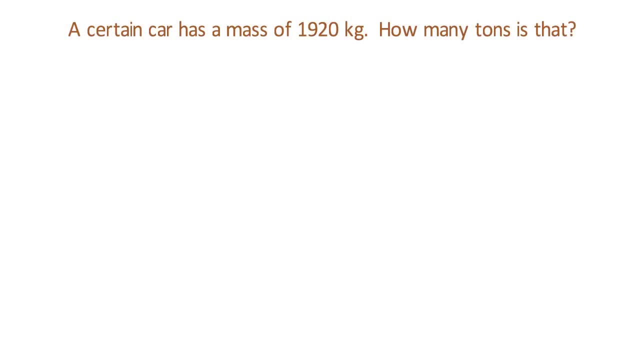 conversion factor before we can solve this. but this time we need two conversion factors: One to convert from kilograms to pounds and another to convert from pounds to tons. So this is going to be a two-step problem. We start the problem by writing down the quantity from the question: 1920 kilograms. 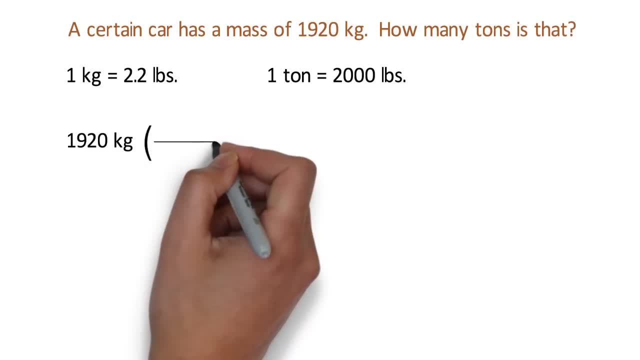 And then we multiply this by a fraction. The two numbers that go in the fraction come from one of the conversion factors. But what goes on the bottom? Because we are starting with kilograms. we write 1 kilogram on the bottom of the fraction so that we can cancel out the kilograms, Next the other. 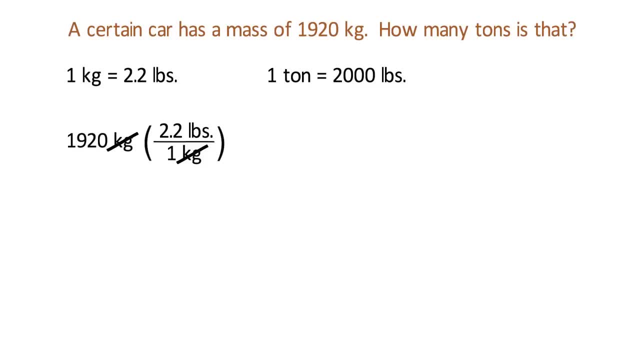 half of that same conversion factor- 2.2 pounds- has to go on the top. The kilograms cancel out, leaving us with pounds as the units of our answer. When you do the math in your calculator, simply multiply the number 2.2 and the other half of the same conversion factor- 2.2 pounds. 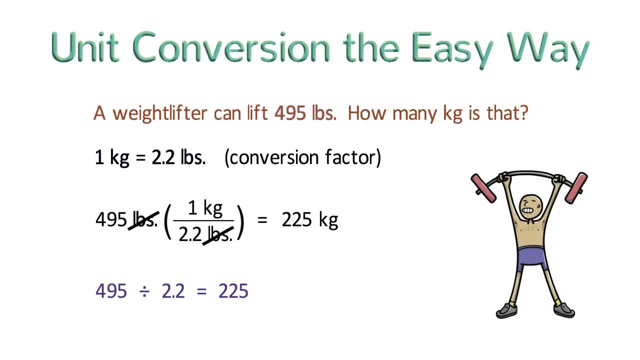 final answer, therefore, is 225 kilograms. There is one more thing that we should notice about this problem: The fraction 1 kilogram over 2.2 pounds actually equals 1, because 1 kilogram equals 2.2 pounds. In fact, any. 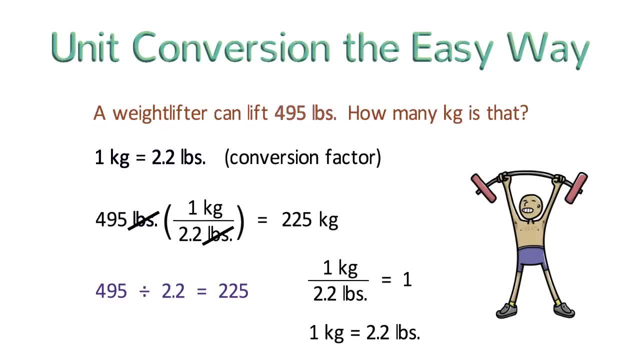 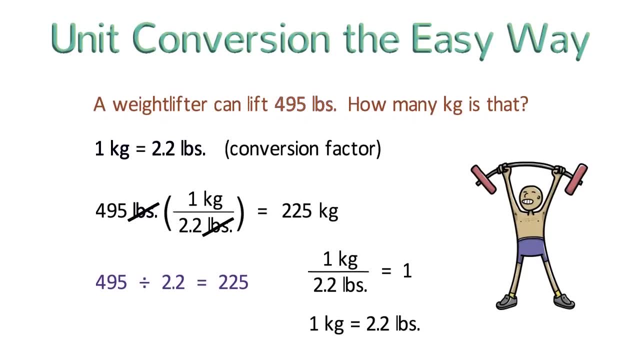 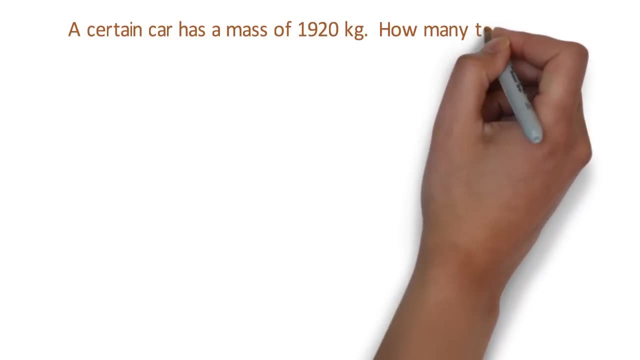 time we do unit conversion, we are simply multiplying our initial quantity by a conversion factor fraction that equals 1.. Okay, Now that we are experts at this technique, let's try a slightly harder problem. A certain car has a mass of 1,920 kilograms. How many tons is that? Just like always, we need a 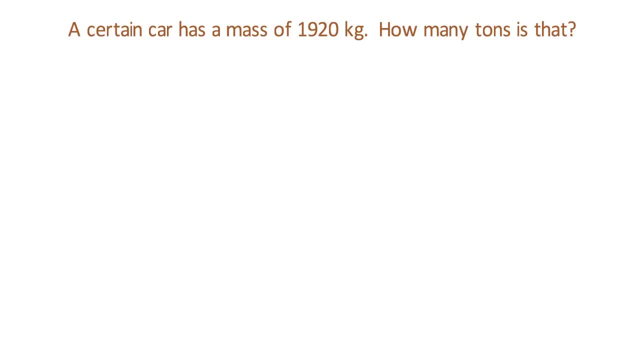 conversion factor before we can solve this. but this time we need two conversion factors: One to convert from kilograms to pounds and another to convert from pounds to tons. So this is going to be a two-step problem. We start the problem by writing down the quantity from the question: 1,920 kilograms. So we're going to start the problem by writing down the quantity from the question: 1,920 kilograms. 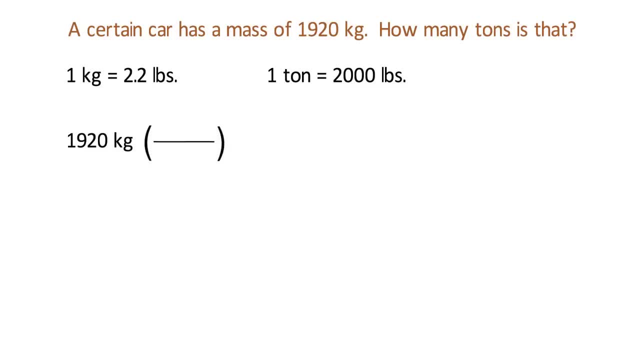 Then we multiply this by a fraction. The two numbers that go in the fraction come from one of the conversion factors. But what goes on the bottom? Because we are starting with kilograms, we write 1 kilogram on the bottom of the fraction so that we can cancel out the kilograms. 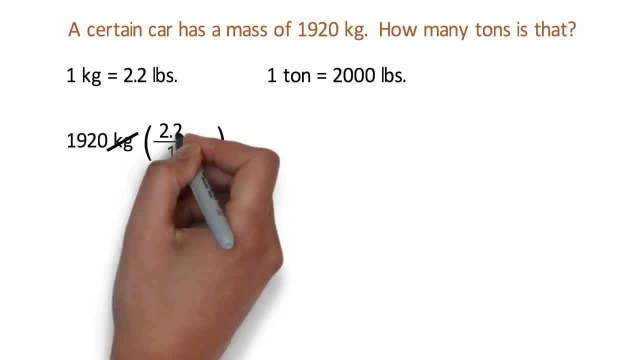 Next, the other half of the same conversion factor, 2.2 pounds, has to go on top The kilograms. cancel out, leaving us with pounds as the units of our answer. When you do the math in your calculator, simply multiply 1,920 by 2.2.. This time we are multiplying the numbers because the one of the conversion factor 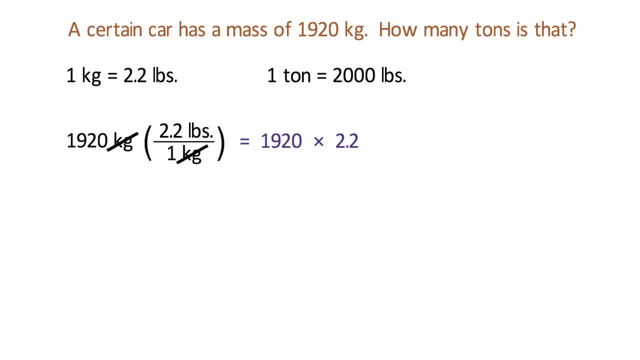 is on the bottom of the fraction. Our calculator tells us that the answer is 4,224 pounds, But we're not done yet. We still need to convert the pounds to tons. The second step works exactly the same way. First we write down the number that we want to convert, that is, 4,224 pounds, and then we 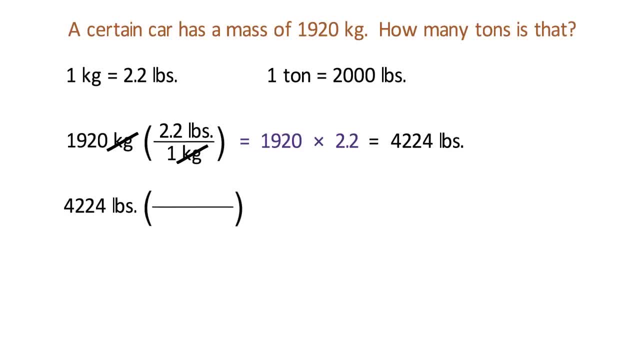 multiply this by a fraction. We want to have pounds in the denominator of the fraction so that we can cancel out the pounds. But which pounds do we choose? 2.2 pounds or 2,000 pounds? Remember that we want to convert to tons, so we choose the conversion factor between pounds and tons. 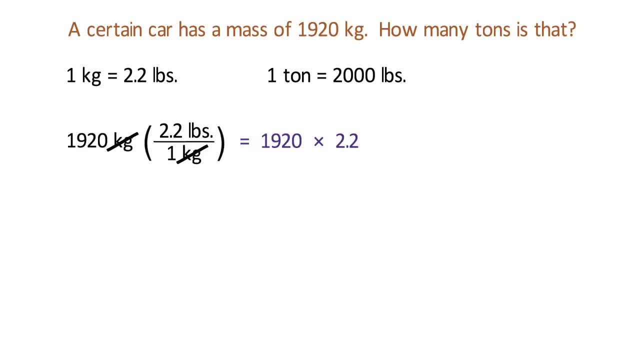 1,920 by 2.2.. This time we are multiplying the numbers because the 1 of the conversion factor is on the bottom of the fraction. Our calculator tells us that the answer is 4,224 pounds, But we're not done yet. We still need to convert the pounds to tons. The second step works exactly. 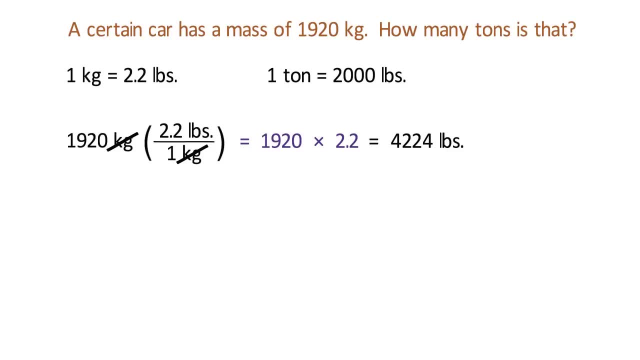 the same way. First we write down the number that we want to convert, that is, 4,224 pounds, and then we multiply this by a fraction. We want to have pounds in the denominator of the fraction so that we can cancel out the pounds. But which pounds do we choose? 2.2 pounds or 2,000 pounds? 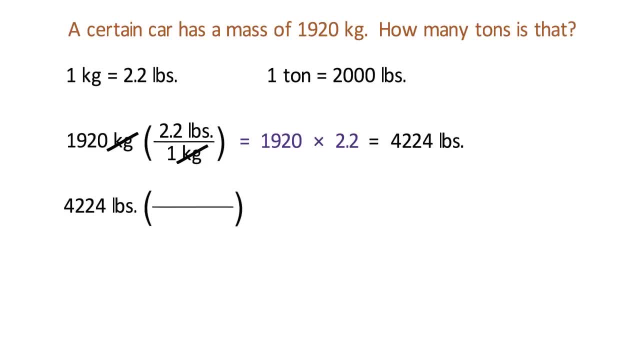 Remember that we want to convert to tons. so we choose the conversion factor between pounds and tons. We write 2,000 pounds on the bottom and 1 ton on the top. Our pounds cancel out and we are left with tons for the units of our answer. In our calculator we type 4,224 pounds. 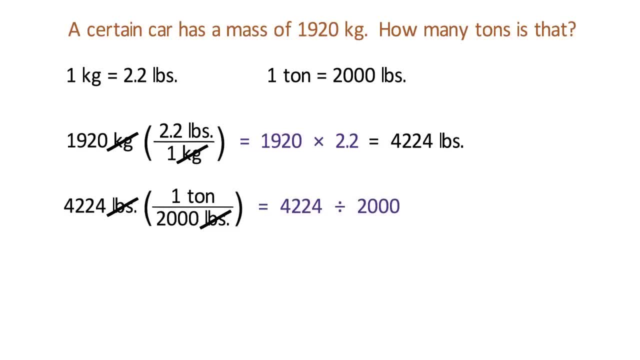 4,224 divided by 2,000, because the 1 is on the numerator of the fraction, Our final answer works out to be 2.11 tons. Okay, we got the correct answer, but it turns out that there is an even better way to solve problems that involve multiple conversion factors. 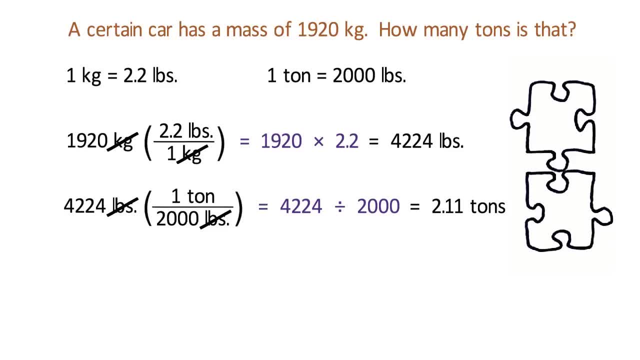 Rather than solving this in two separate steps, we can combine those steps into one step with two conversion factors. Check this out Once again. start the problem by writing down the quantity that you want to convert. Multiply the number that you want to convert by 2.2 pounds. 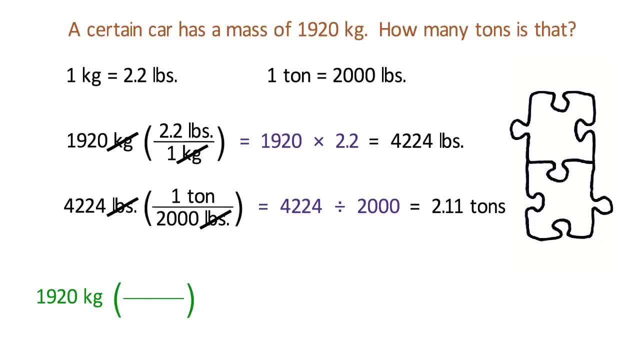 We do this by conversion factor fraction, putting what you want to cancel out on the bottom and what you want to convert it to on the top. Notice that so far, this is exactly the same as the first step we just did. However, instead of solving this as it is, we're going to multiply it by another. 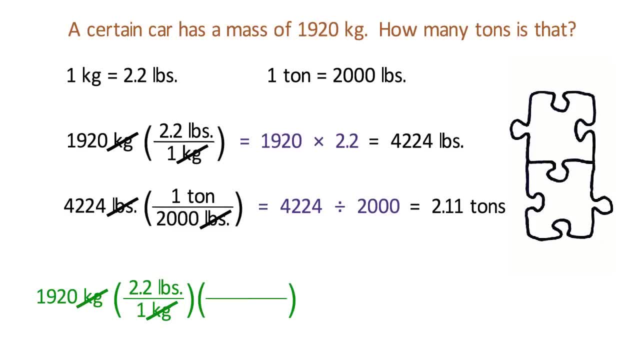 conversion factor fraction. We now need to cancel out the pounds that are left on top, so we put 2,000 pounds on the bottom. We chose 2,000 pounds rather than the 2.2 pounds because we ultimately want to convert the quantity to 2.2 pounds. We now need to cancel out the pounds that are left on top, so we 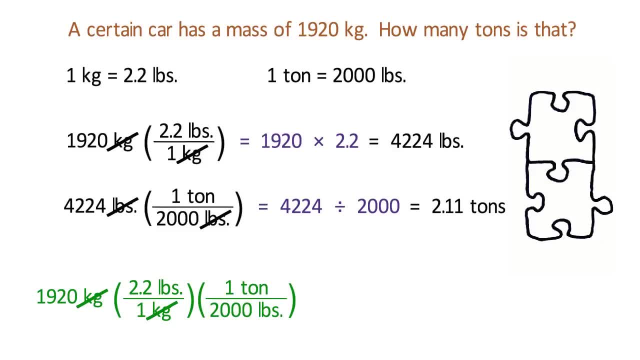 choose 2,000 pounds rather than the 2.2 pounds. This gives us tons as our remaining units on top, while all the other units cancel out. We then proceed to calculate from left to right. If the one is on the bottom, we multiply, If the one is on the top, we divide. So we multiply 1,920 by 2.2.